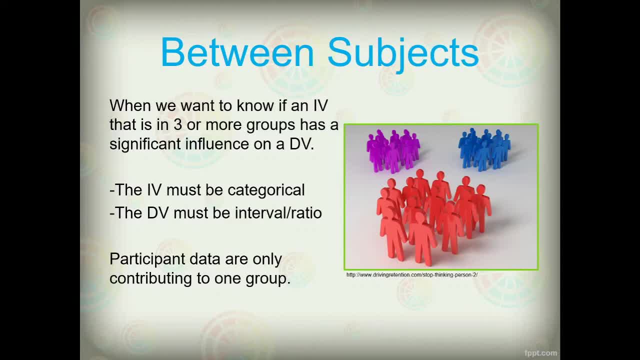 different from group to group to group. That's right. it's three or more groups. So we want to know if the independent variable, that is, in three or more groups, has a significant influence on the dependent variable. That's the general gist of an ANOVA. The independent variable has to be categorical: two or more groups, The dependent 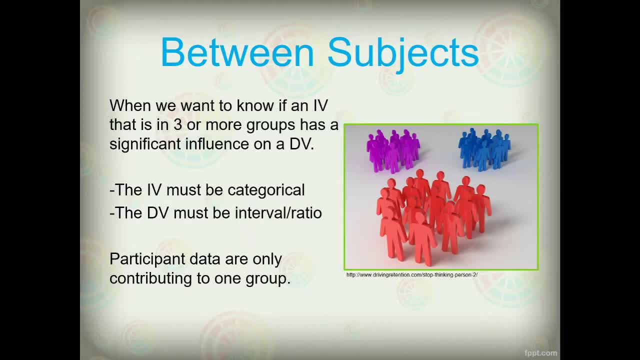 needs to be either interval or ratio, it needs to be a continuous and for a between subjects design, each participant will only contribute data to one of the groups, not all three of the groups. so each subject or respondent or participant will only be contributing information to one group. that's what. 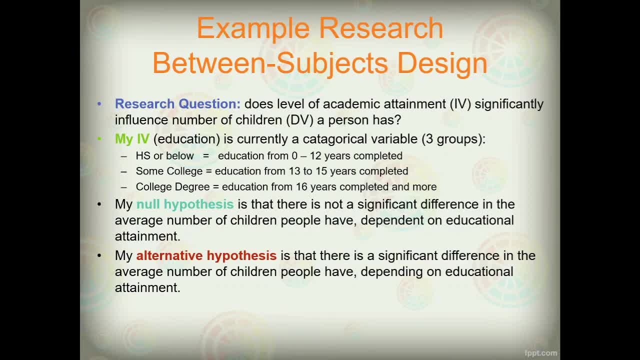 makes it a between subjects design. so let's come up with an example here. let's look at one. let's say the research question is wondering: does the level of academic attainment, the independent variable, significantly influenced- number of children or dependent variable that a person has? so it is the level of. 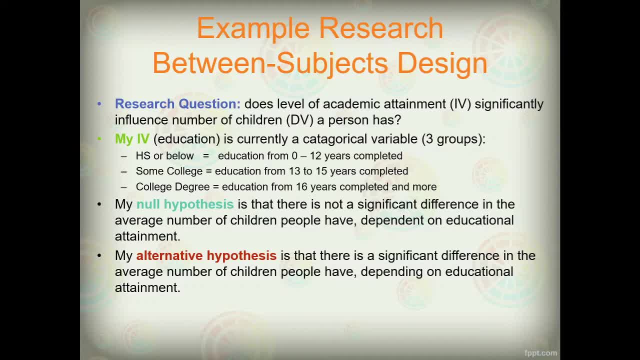 academic attainment significantly influenced number of children a person has. the independent variable, which would be education or academic attainment is currently it's a categorical variable, because sometimes, of course, can be a continuous variable, but we're looking at data that actually had it divided into three different groups: high school or below some college. 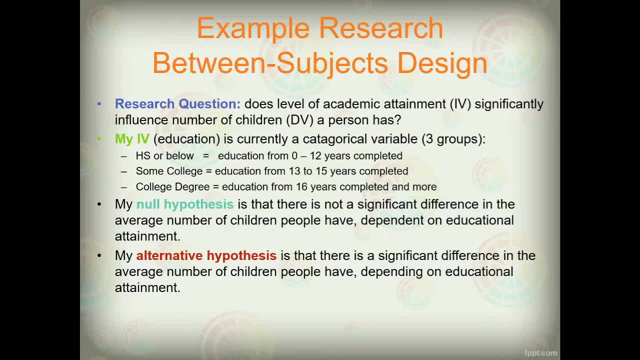 or college degree. so the null hypothesis is that there's not a significant difference in the average number of children people have dependent on their educational attainment. and the alternative hypothesis, which is also known as the research hypothesis or scientific hypothesis, is that there is a significant difference in the average number of children people have. 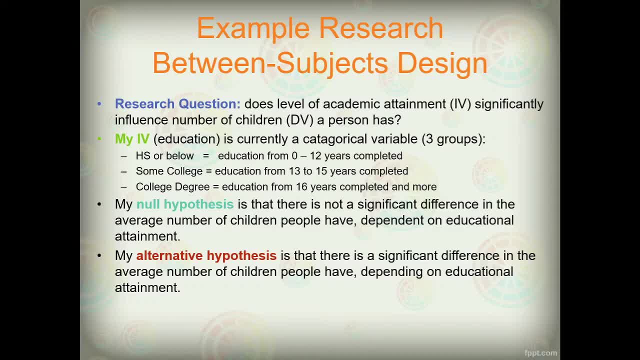 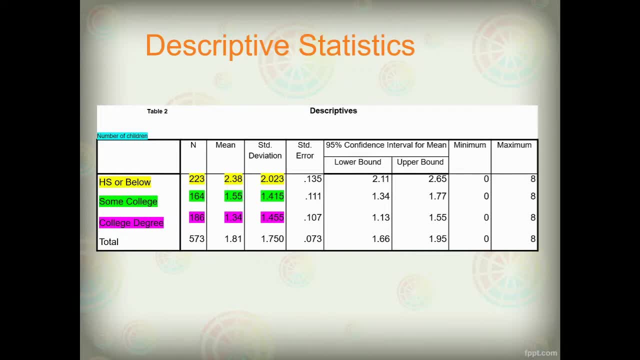 depending on educational attainment. so we've run it in SPSS and here's one of the first output boxes we see. these are our descriptive statistics and this is going to tell us about our total and our individual groups. and I'm really interested in the individual groups. so the group of high school or below here. 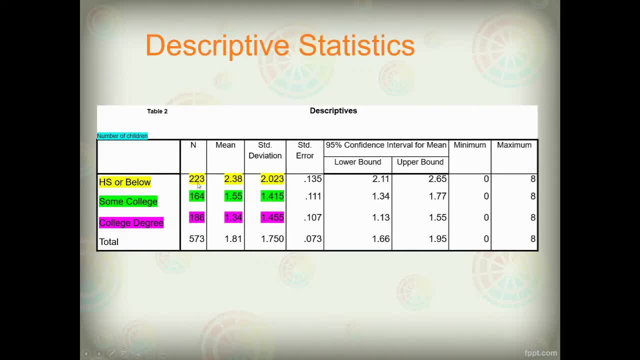 highlighted in yellow is our count. so we see we had 223 participants in this group. they had an average number of children of 2.38 with a standard deviation of 2.023, and then some college. we see there's 164 people with an average of 1.55 number of: 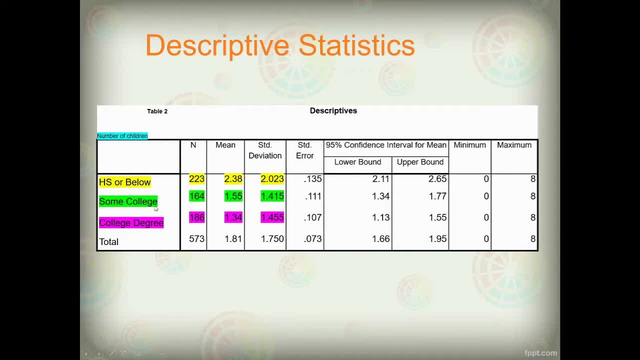 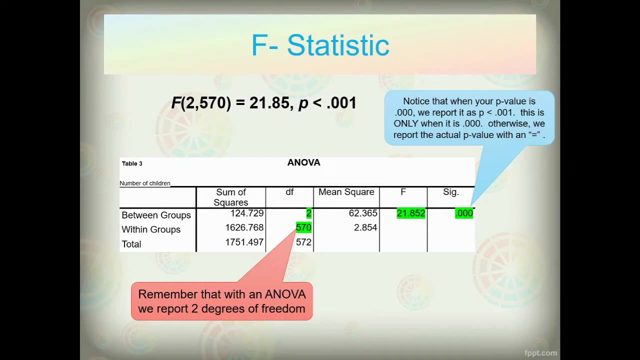 children and a standard deviation of 1.45, and so on. college degree: 186 people, 1.34 children, 1.45 standard deviation and these are important and we're going to need these to write up later. but we also got another output box and it is: 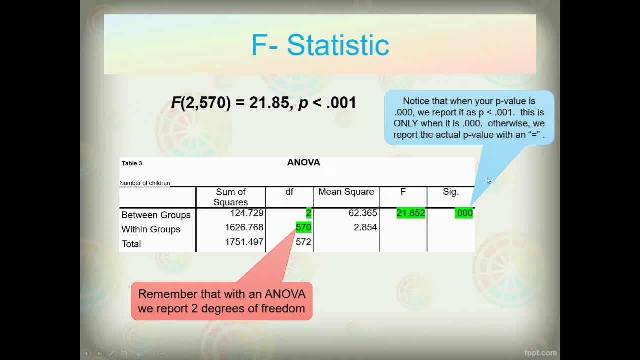 our F statistic. well, the output box. it's not quite in the proper format or order, but we can find all the information in here. first thing that we want to look at is our significance value, and we see a significance value of point zero, zero, zero. that means this is our p-value and it 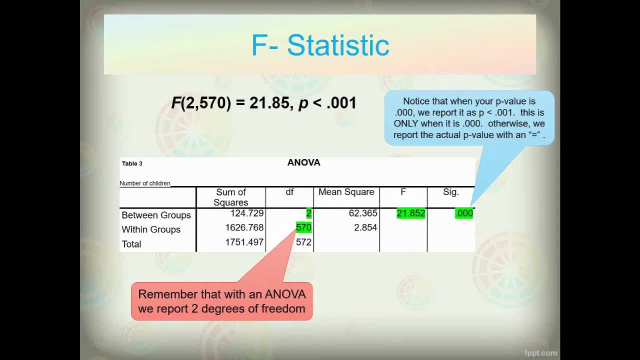 is below the alpha level of 0.05, so this is significant. we are finding that there is a significant difference in the number of children that each group average is that each group has averaged. unfortunately, we don't yet know which group is different than which group. we 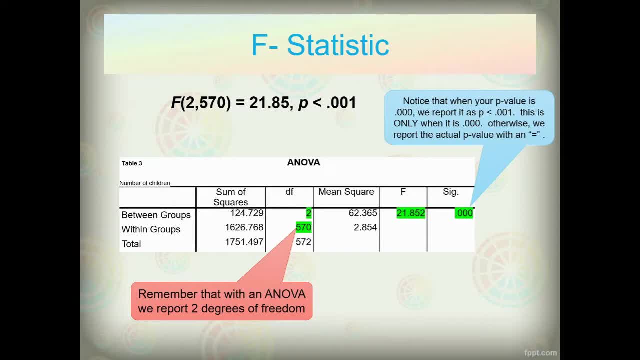 just know that somewhere between the three groups there is a significant difference in the number of children. on average, that group has now little side note. whenever SPSS spits out a significance value of 0.00 zero, you always want to report it as less than 0.001, and this is because 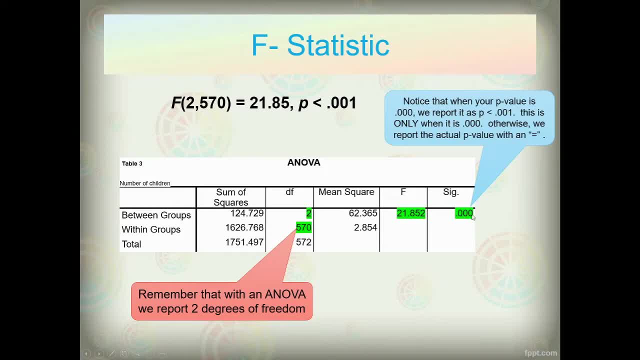 in reality, this number is actually 0.000002942 or something. it's a very, very small number. it usually does not equal 0. I don't think I've ever seen it equals zero. however, there is a small number back there there behind it, So we just write that it's less than 0.001 and that tells the reader exactly what. 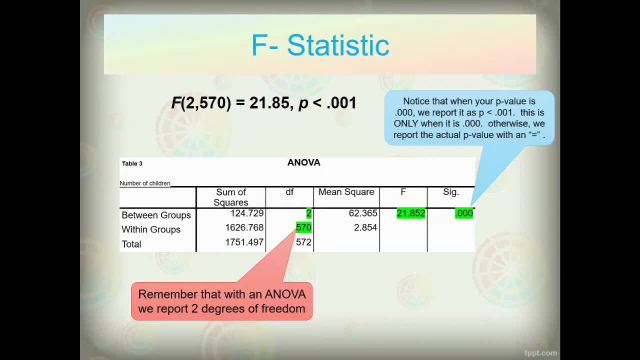 they need to know. Otherwise, if it were any other number, you're going to report it as a p equals and the exact number that it is. The only time we ever change it is when it's the three zeros. Here's our f statistic, which is 21.85, and then, for our degrees of freedom, we're going to report both. 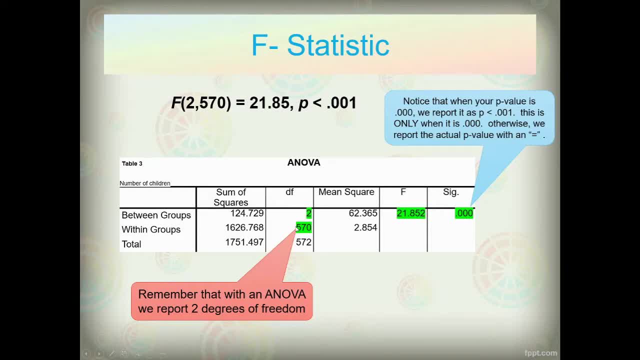 our between groups degrees of freedom and our within groups degrees of freedom. Remember when you were first learning about ANOVA- and ANOVA is actually a ratio, that the f statistic is actually a ratio and it's looking at the between groups over the within groups. So we always want to report. 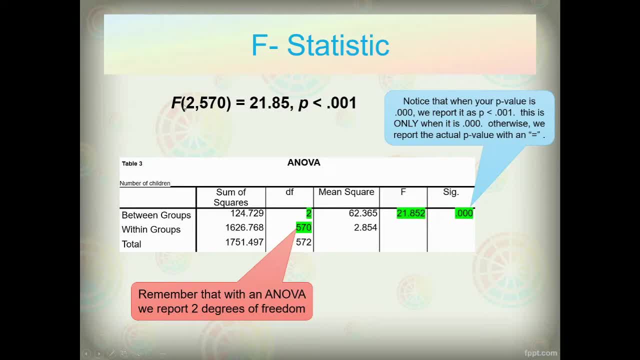 for both and when we report it. here's how we're going to write it up. This is how the APA format. so we have our capital F for our f, statistic, and, and it is italicized, as is the p, because all Latin statistical abbreviations should be italicized. 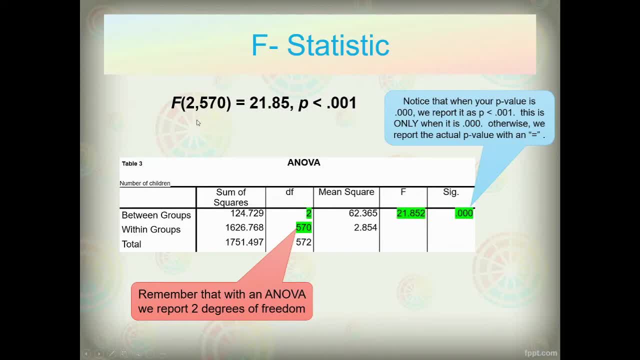 There's no space. and then there's the degrees of freedom, which are 2 comma 570.. Then there is a space and an equals and a space. Now always keep in mind our equal signed are greater than or less than signs. We treat these like words. They should have a space before it and a space after it, just. 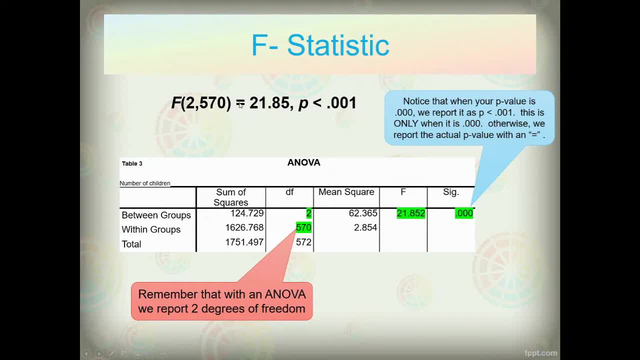 like a word would. So we have our f, our degrees of freedom equals, and this is our, actually our actual f statistic. That's our cheers, and then it has a comma and a felony, And that's our entire f statistic. Let's go to the next slide and see what we're up against. Ah, I know what's coming next, So we know. 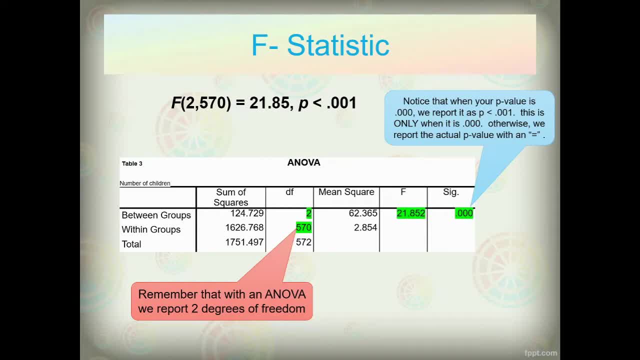 right now, when we think of our f statistic, We have a p value less than 0.01.. That means it's significant. There is a significant difference in the average number of children that each group has two and group three. group one and group three, we don't know. so let's run what we call a post-talk. 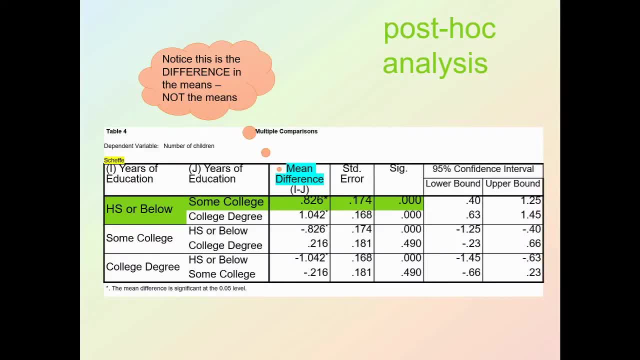 test and that is an after-the-fact test that we're going to run. we actually ran the cheffy test and the reason why we ran a cheffy and not a tuki: we ran a cheffy because, if you recall the number of 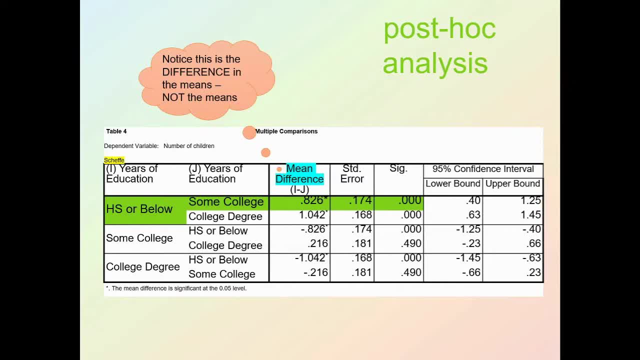 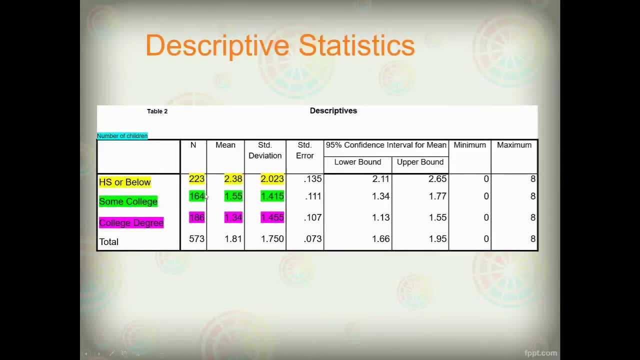 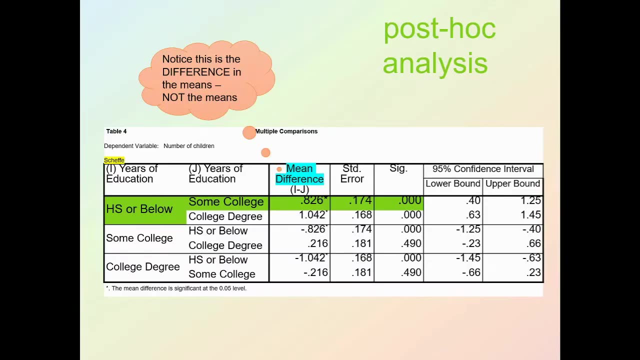 participants that we had in each of our groups. let me see if i can go back without nope, i went the wrong way. the number of participants we have: we have 223, 164 or 186. they're not all the same. so that's why we're going to run a cheffy. if we had the same number of participants, if each of the 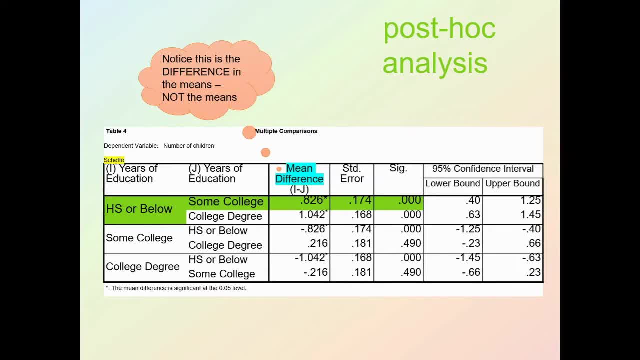 groups were evenly distributed for their count, then we would run a tuki. so i ran a cheffy and what this is is: you see a matrix here. we're looking at high school or below and we're comparing or not not really comparing. we're running a test to see. there's a small test seen here. if there. 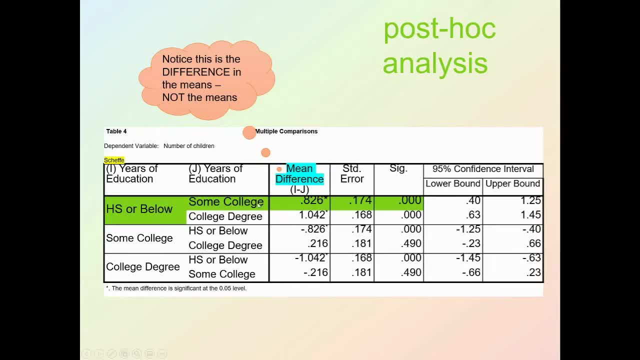 is a significant difference between high school and below in some college, and here is going to be those results. or high school and below and college degree, and here's going to be their results. then we go down one and we see some college to high school or below. 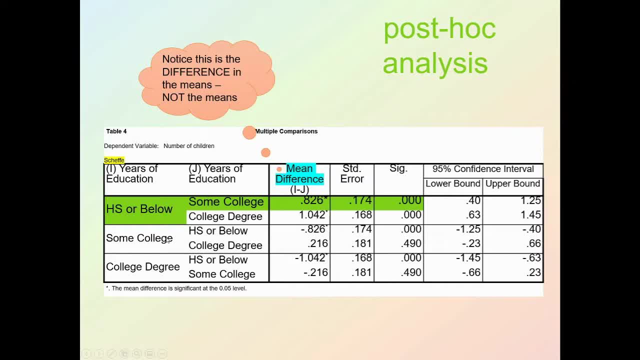 and then we see some college to college degree, so there's a matrix. we're going to have duplicates. we have some college to some college, some college to high school, so these two are going to be the same. we have some college to college degree and we have college degree to some college, so we have 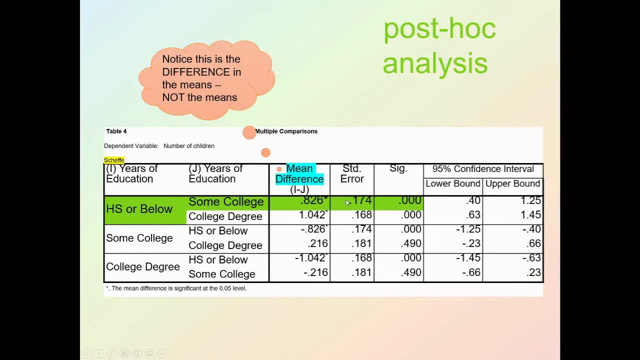 duplicates. we have three results, but with spread out over six rows, so we have a duplicate of all three results. now you want to be careful not to when you're reporting your descriptive statistics. you don't want to get your means from here. this is actually the difference in means. 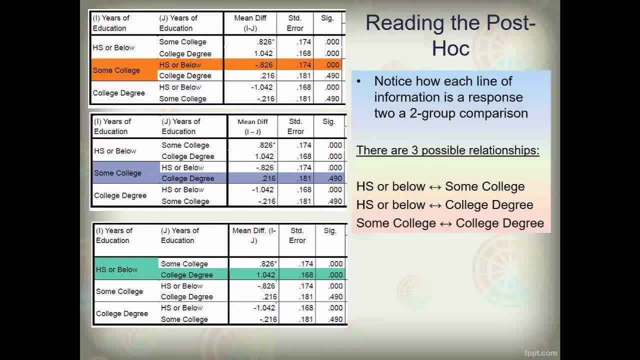 so you just want to keep that in mind, but let's take a look at all of these at the same time. so here are the three things that we need to look at, the three different relationships that we want to test, to see which ones are or are not significantly different from each other. 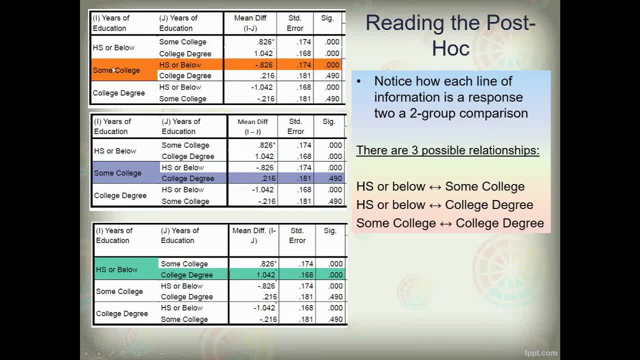 we want to know if some college to high school and below are significantly different from each other, and they are. we want to know if some college to college degree are significantly different from each other, and they are not. 0.490 is not below 0.05, so 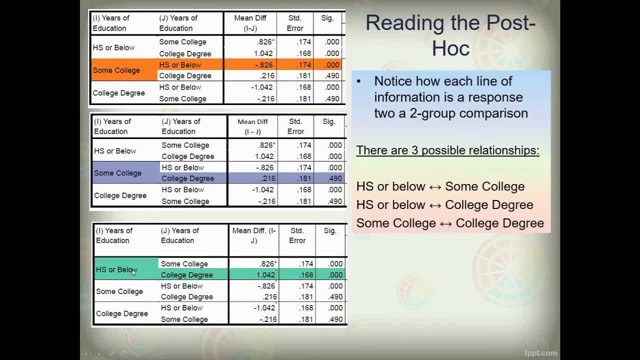 they are not significantly different and we want to know if high school or below and college degree are significantly different from each other and they are, so high school or below and college degree and high school or below and some college are both significantly different from each other, as we can see. 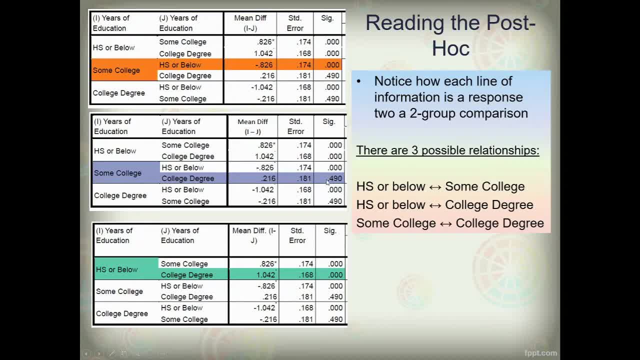 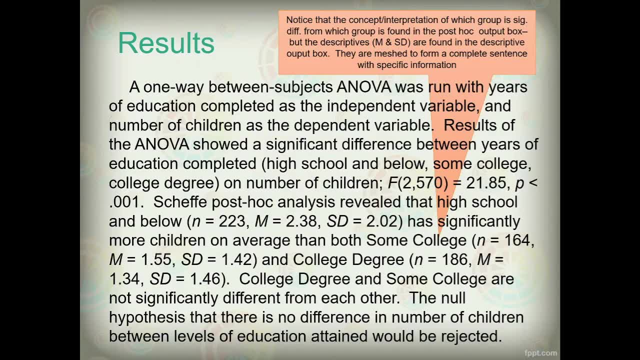 some college and college degree are not significantly different from each other. So how are we going to write this up? Well, let's go forward and figure that out. I'm going to go ahead and read through this and then we're going to break down all the parts of it. 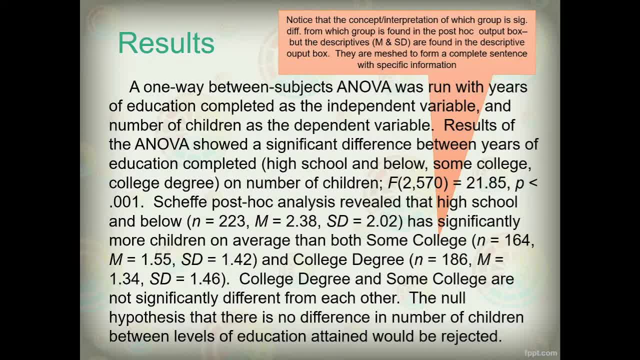 Now, when I read through this, this is how I do it, But the first time that I read through results, I don't read what's in the parentheses. It kind of gets at my brain a little too much. So I just want to get the concepts down and then I can go back and look at what's in the parentheses. I can. 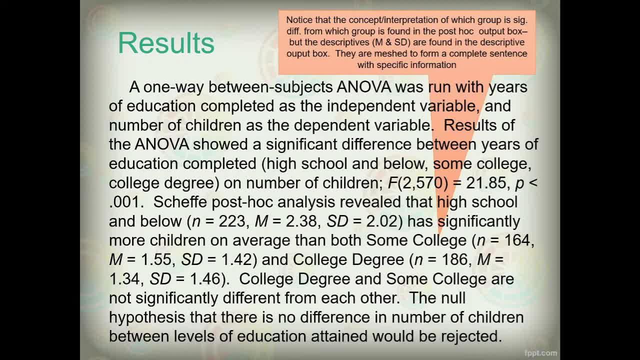 go back and look at the details. Those are details, but the concept should be there without that, So I'm going to skip over some of this stuff. A one-way between subjects ANOVA was run with years of education completed as the independent variable and number of children as the dependent. 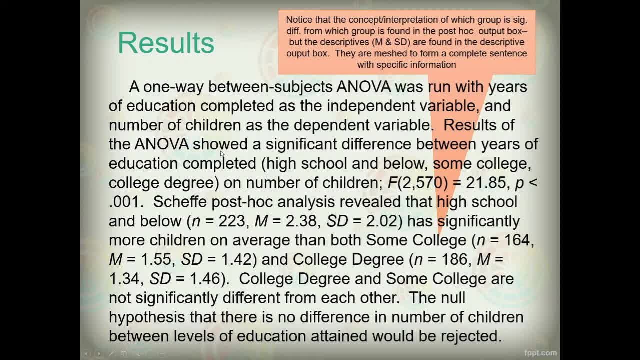 variable Results of the ANOVA showed a significant difference between years of education completed on the number of children. NRF Sheffy post hoc analysis revealed that high school and below has significantly more children on average than both some college and college degree. 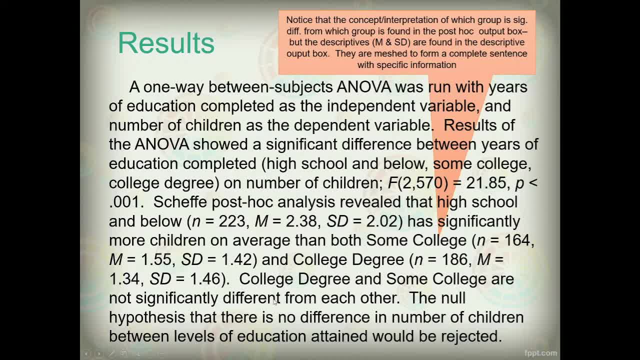 College degree and some college are not significantly different from each other, The null hypothesis that there is no difference in number of children between levels of education attained would be rejected. Okay, that kind of made sense, So let's break it down. How was it that I wrote this up? And let's 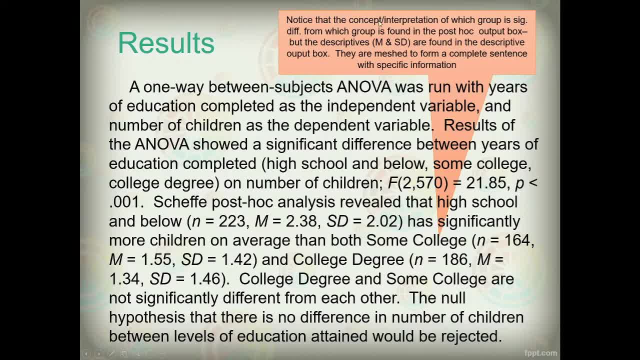 see what's the notice say here That the interpretation or the concept of which group is significantly different from which group is found. Notice that the concept or interpretation of which group is significantly different from which group is found in the post hoc output box. but the descriptives, the mean and standard. 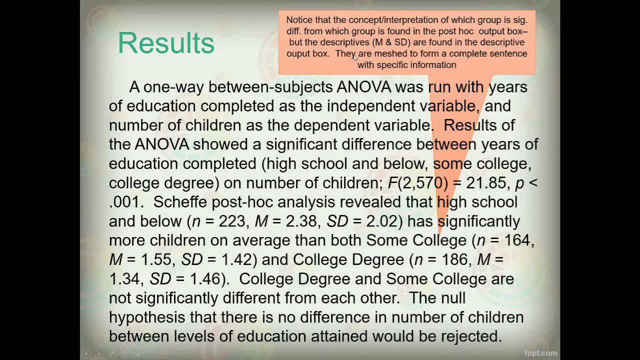 deviation are found in the descriptive output box. so we need to kind of mesh those two output boxes together into this sentence. we want to drop our descriptives. as you can see, this comes from our descriptive box, but it's kind of combined into where we're talking about the post hoc. okay, let's go forward. 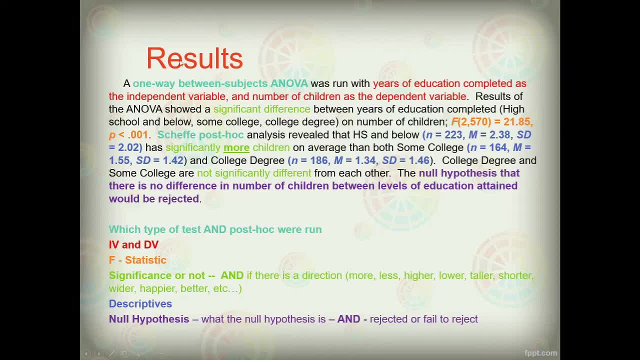 so here is the exact same paragraph but I've color-coded it for us. so we want to see in this color we see which type of test and post hoc tests are run. so a one-way between subjects ANOVA tells us what kind of test we ran was run with. 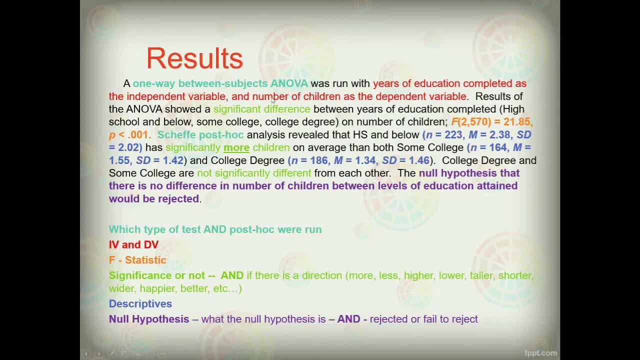 years of education completed as the independent variable and number of children as the dependent variable. so that clearly states what the independent variable and dependent variable are. results of the ANOVA showed a significant difference and this is very important. you always have to say whether it's significant or not significant. 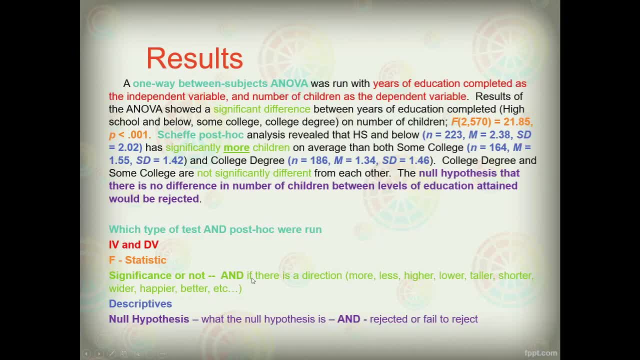 and if there's a direction between the two, which you'll find, we'll see later- then you always want to report that as well, just like we did in the t-test. so back to here. results of the ANOVA showed a significant difference between years of education completed which included high school and below some college. 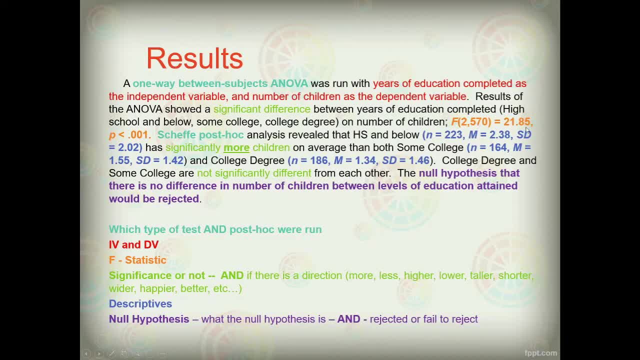 college degree a number of children, and here's our F statistic. when we wrote this up once the F2570 equals 21.85, with a p-value of less than 0.01. a Sheffy post hoc analysis revealed that high school and below had significantly more children on. 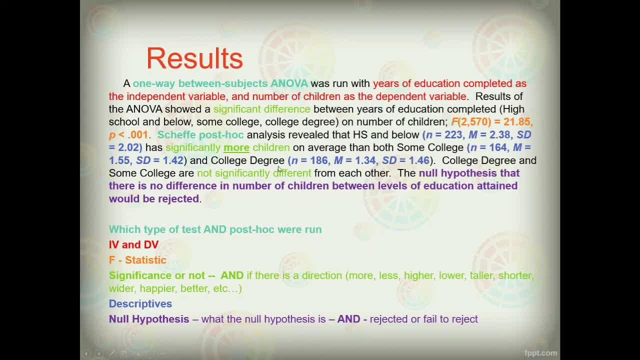 average than both some college and college degree. so I added the significantly more children, not significantly different. we can look at the average and see that this average was 2.38 children where this average was 1.55 and this average was 1.34. so we 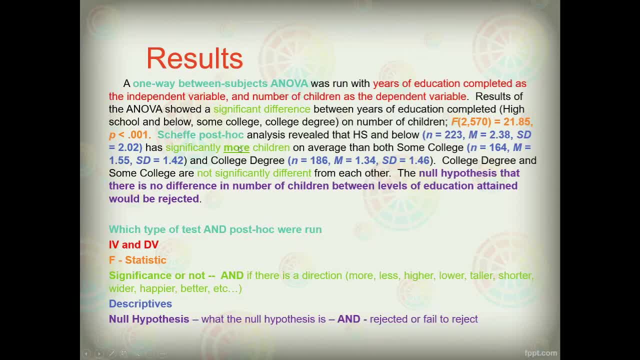 know that high school and below had significantly more children. this is what I mean by adding a direction. we also note that this is where we added all of our descriptive statistics. we've got our number and our number has a lowercase end, and that's because we use a capital N, with a total population and a. 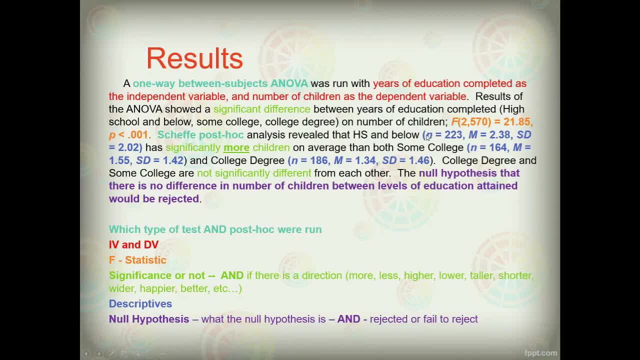 lowercase N when it's a sub population. so our total population was 500 and something, 223 plus 186 plus 15, 164 or- yeah, I'll never get this fast enough- 580, something, maybe. anyway, we use a lowercase N because these are all three subpopulations. we add the mean and the 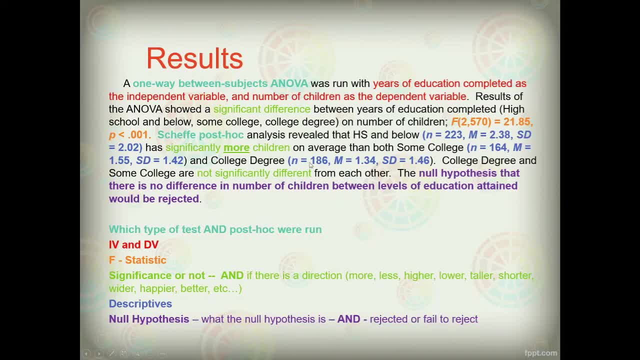 standard deviation and this is a really good format. this is nice APA for format. we have our Latin statistical abbreviations are italicized, we have spaces before and after our equal signs separated by commas. perfect, and then sorry. and then we discuss the fact. so through here we've discussed two out of 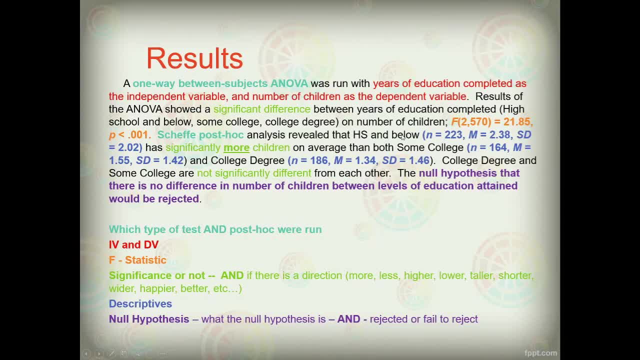 the three relationships that high school and below is significantly has significantly more children than some college. that's one relationship. and then high school and below and college degree, that's a second relationship. but our third relationship, college degree and some college, are not significantly different from each other. we had to discuss that as well. the null: 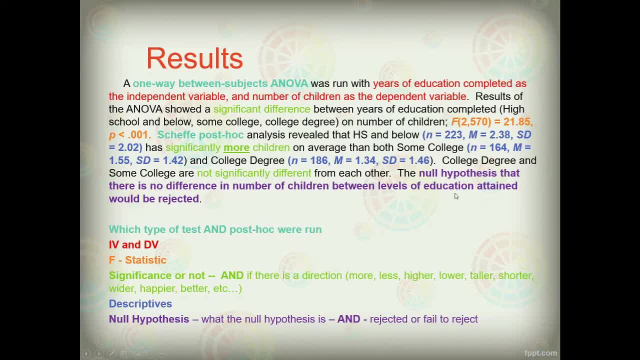 hypothesis that there is no difference in number of children between levels of education attained would be rejected. and this is when we address the null hypothesis. you always, always want to restate the null hypothesis when you're doing homework. it seems like you just wrote it like a paragraph ahead of this. 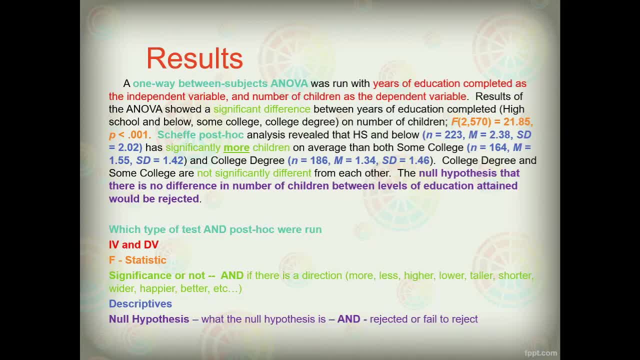 but when you're actually writing a paper, you'd probably talked about the null hypothesis a couple of pages ago, so you always want to restate it when you're discussing whether you're going to reject it or failing to reject it, because the reader oftentimes has it. it could have gotten a. 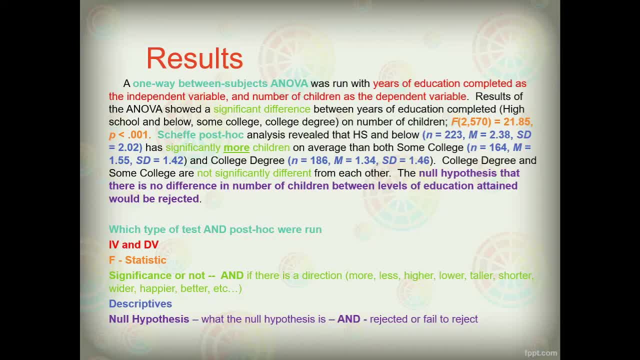 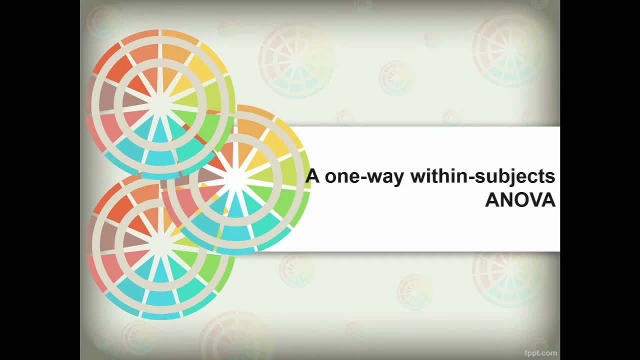 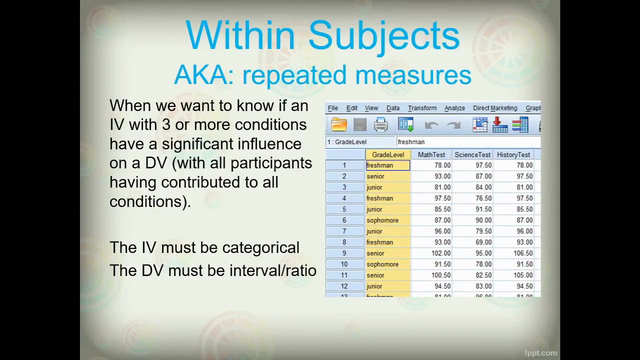 little bit foggy over the pages of information that they've taken in, so you want to present that very clearly for the reader. all right, so let's move on to our one-way within subjects ANOVA. here we go. so within subjects ANOVA is also known as a repeated measure, ANOVA and this 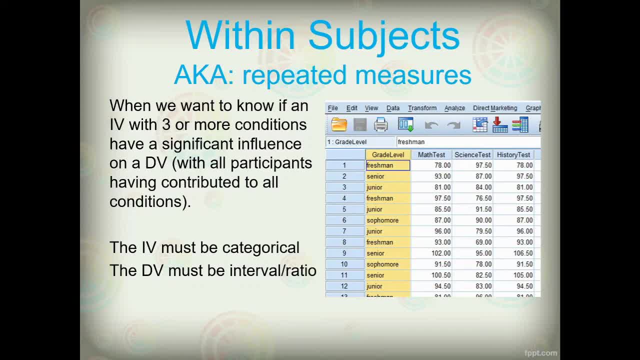 is when we want to know if the independent variable with three or more conditions have significant influence on a dependent variable. now, all of the participants having contributed to all conditions, that's very, very crucial. that's what makes that a within subjects. so, with the between subjects, participants only contributed to one. 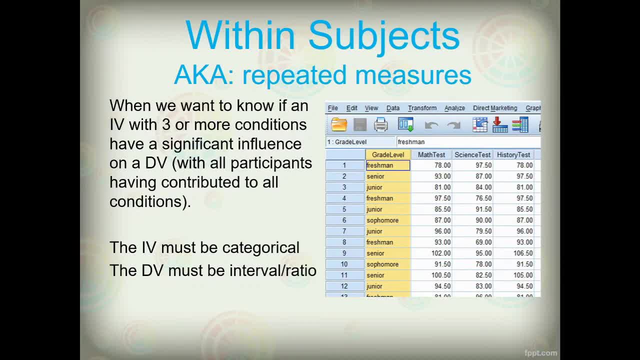 condition or one group. For this one we have the participants contributing, so one participant is going to contribute to all three groups. The independent variable still needs to be categorical and the dependent variable needs to be interval ratio. So it's the same setup. 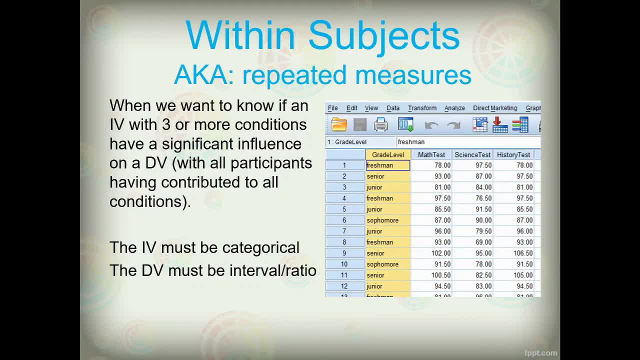 but it's a matter of how often the participant is contributing to the data And whoops, if you want to take a peek at this. So here's a good way to kind of visualize it in SPSS. but we can see that this is a participant. This participant was a freshman. They took 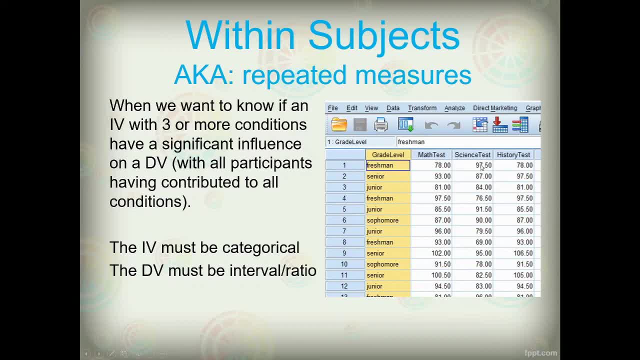 a math test, They then took a science test, They then took a history test. So one person, or one participant or one respondent, one subject contributed to all three groups And will be accounted for in all. three of the group means OK. So our example is: let's 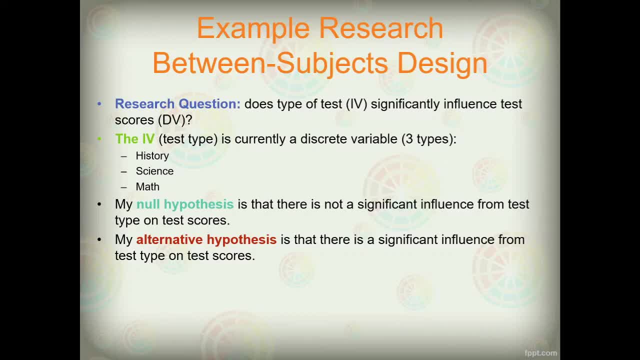 look at a research question of: does the type of test, which is our independent variable, significantly influence test scores, our dependent variable? So the independent variable currently a discrete variable or categorical variable? There's three, with three conditions. We have history, science and math And the null hypothesis is that there is not a significant 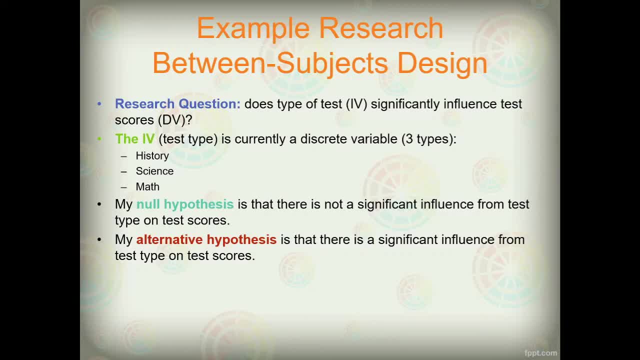 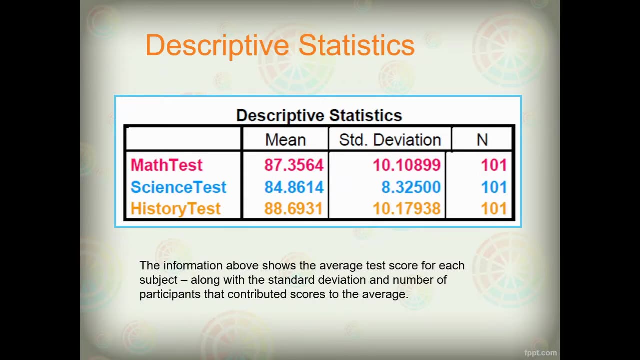 influence from test type on test scores. And the alternative, or research hypothesis, is that there is a significant influence from test type on test scores. We get our descriptive statistics once we've run it And we see here that math test has a mean of 87.35, standard. 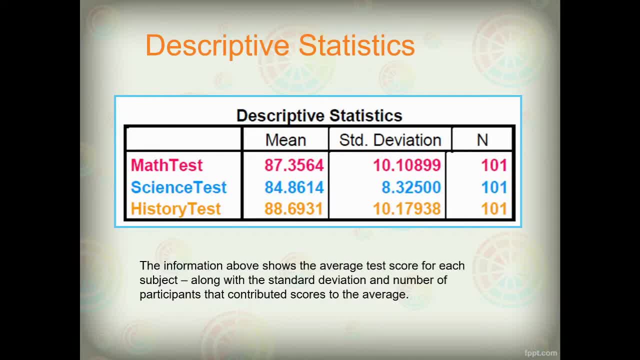 deviation of 8.51, and the question is whether the test type is descriptive or not. So here's 10 and our number is 101. now that means we had 101 subjects taking the math test. but if you look at the number, you'll note notice that there's 101 subjects that also took the science test. 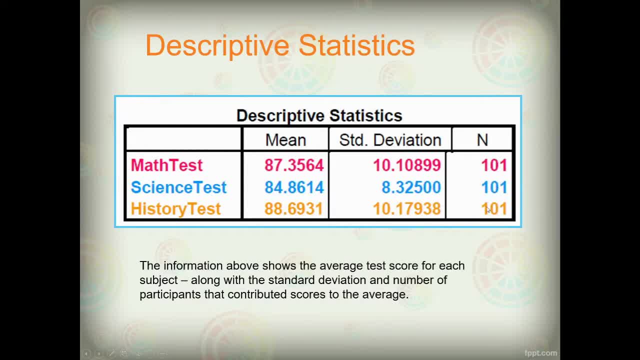 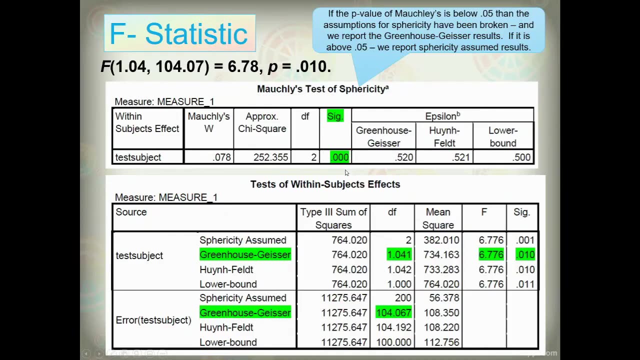 on the history test and keep in mind this is a within subjects design, so these should be all the same participants. the same participants that took this test are going to be the same participants that took the science test and that took the history test. so that's why we're going to test our f. we're also going to get some output boxes that are: 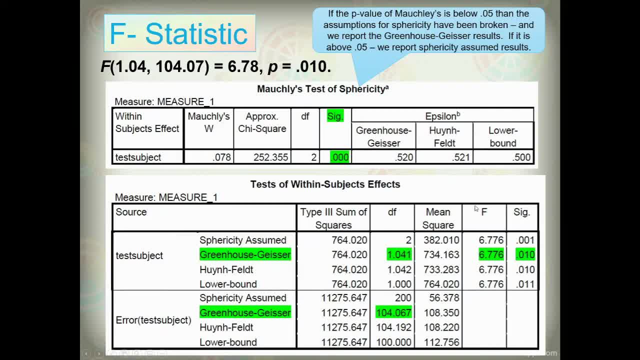 going to give us our f statistic when we look at it. this second box is our test of within subjects effects and this is the one that's going to give us our f. but you'll notice there's a lot of different options to choose from. there's actually four different options that we want to choose from. 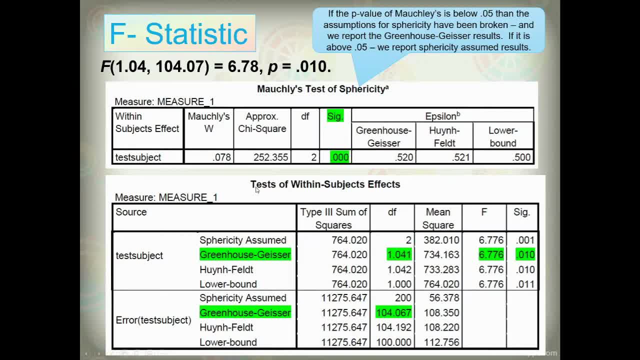 so why do we have all these? well with an ANOVA is whether or not that we've met sphericity, and sphericity is basically saying that the population variances of all possible differences are equal, or that the variances of the difference of the differences are equal. if this is broken, then we need to use a different. 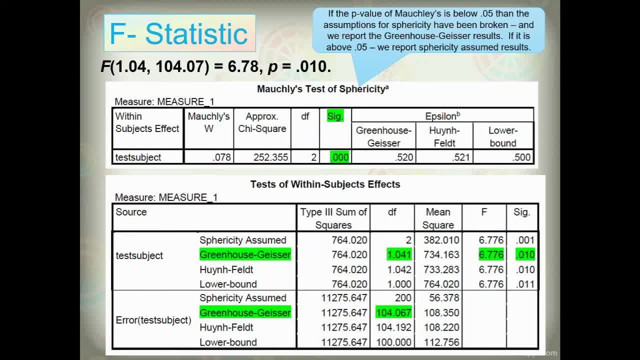 measure. we need to report a different measure which can be a little bit more strict. the calculation is a little bit more strict so that there's not any overestimation of the differences. so we want to look before we choose our f test. we need to look at our 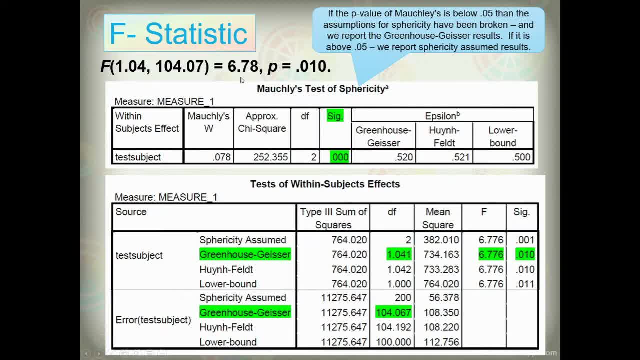 motchley's test of sphericity and this is going to determine whether we have broken the assumption of sphericity or not. so when we look at this, we go straight to significance and we see that it is below 0.05. when a test of an assumption is significant, that means we have broken the assumption. 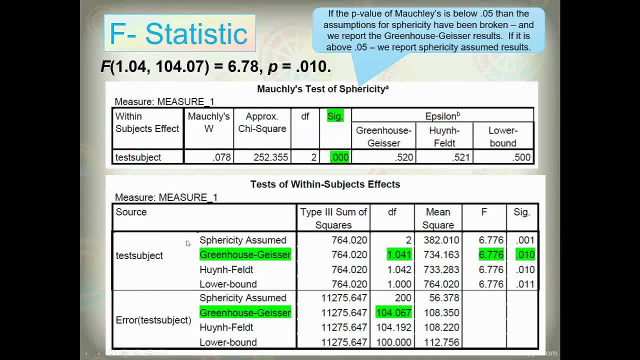 so we cannot use sphericity assumed. we do not assume sphericity because we know that we have broken sphericity assumption. so we're going to use the greenhouse geyser, which is the second line, and we see it for both. so when we 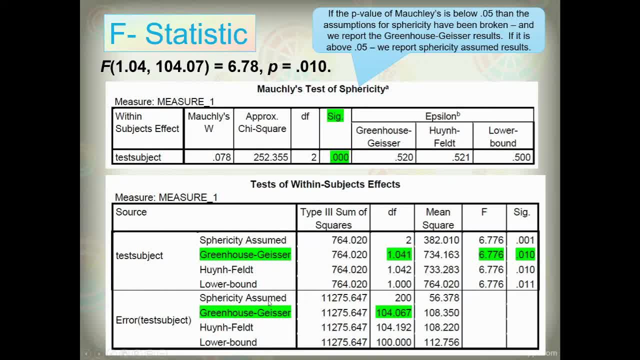 we looked at the ANOVA results, we had to get our two degrees of freedom from between and within. We're going to do the same thing here, but there are just multiple options. So our test subject is more comparable to what we saw earlier on the between subjects and the error or the test. 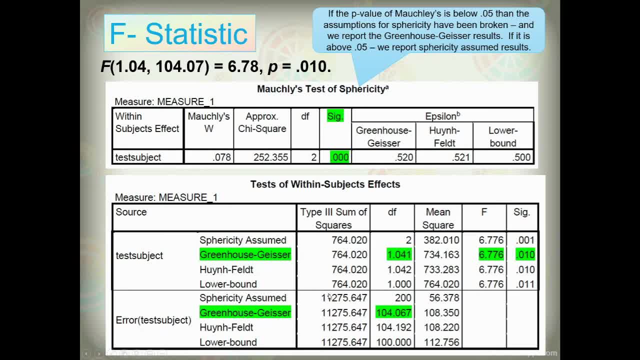 subject would be more comparable to what we see on within. Sorry about that. I was trying to go down the screen, So we're going to look at this one. We see it's below 0.05, and then we're going to take our information. I've highlighted it from the green highlights We're going to use. 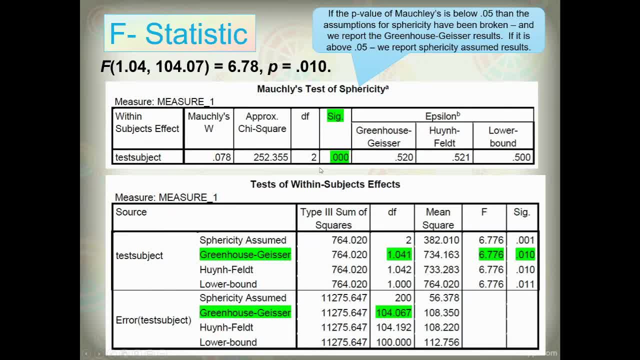 Greenhouse Geyser. So our F statistic, with our degrees of freedom of 1.041 and 104.067, equals 6.78, and our p-value equals 0.010.. Our p-value is below 0.05,, so this is significant. 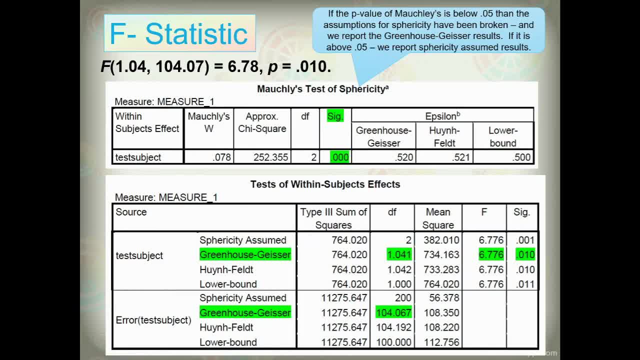 So we know that there's a significant difference in the average test scores between the history test, the math test and the science test. What we don't know is where those differences exist, whether it's between history and science, history and math, math and science or all three. So let's find out where they are. 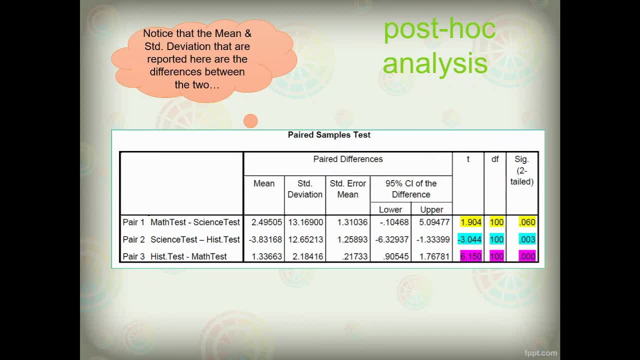 and let's check out our post hoc test, Because we had a within subjects design. we're going to run basically a paired samples t-test- and this is something that most of you participated in a week or two ago, but we're going to run a paired samples t-test. The first pair we're looking at is whether math 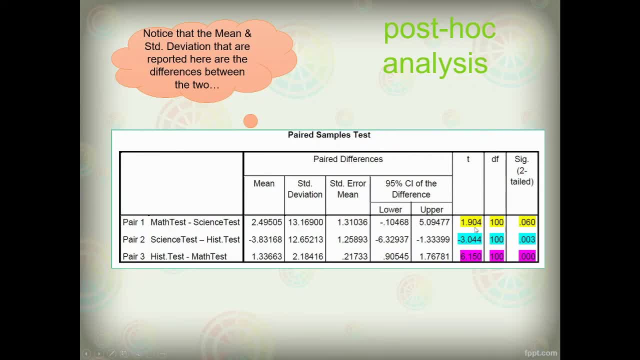 and science tests are significantly different- and we can come right over here- and we can see that they were not significantly different from each other. The science and history test are significantly different from each other and the history and math test are also significantly different. 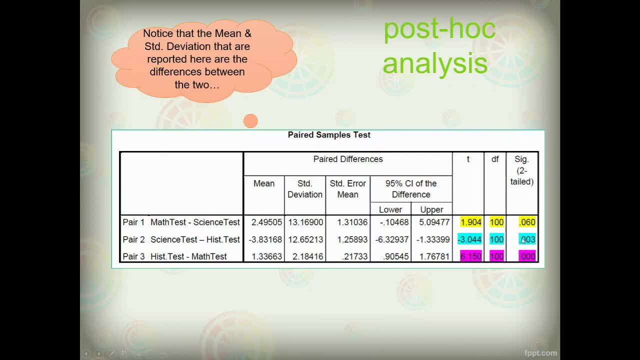 Both of these bottom two are below 0.05, so they are significantly different from each other. Here is our t-score and our degrees of freedom. So when we're writing this up in results, when we're talking about our post hoc, we can discuss the t's, because it's the t values that 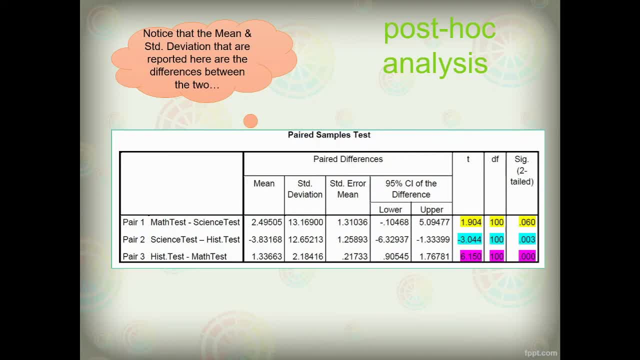 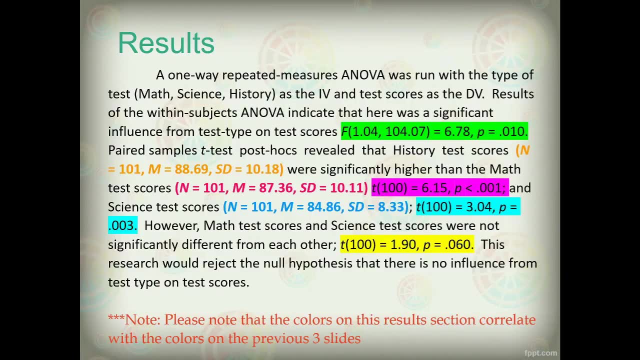 tell us whether or not they are significant. Okay, let's go forward into our test. Preparing our results. A one-way repeated measures ANOVA was run with the type of test- math, science or history- as the independent variable and test scores as the dependent. 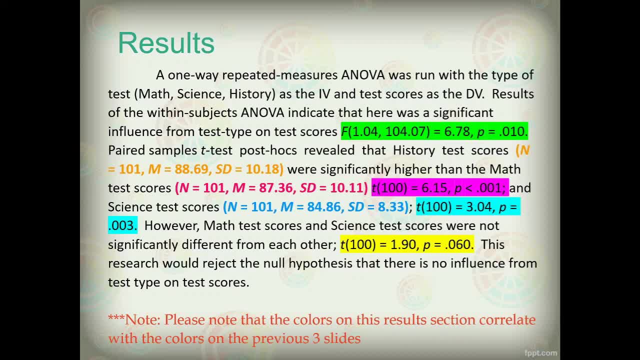 variable Results of the within subjects ANOVA indicate that there is there was a significant influence from test type on test scores. Sorry, I just saw that other typo, That there was a significant influence from test type on test scores. Sorry, I just saw that other typo.